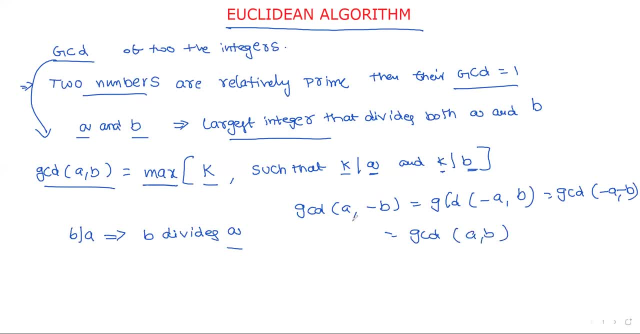 is equal to GCD of a comma b. Whatever the value of, that is sign of the two numbers. always it is considered as mod a comma b. That is, the operation is performed between the positive integers Even though we are using the negative values. the operation is performed between positive integers. And one more thing: 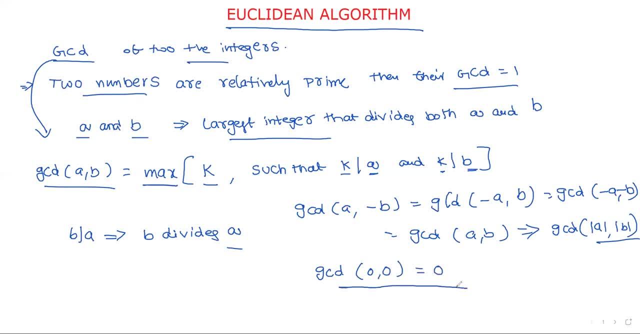 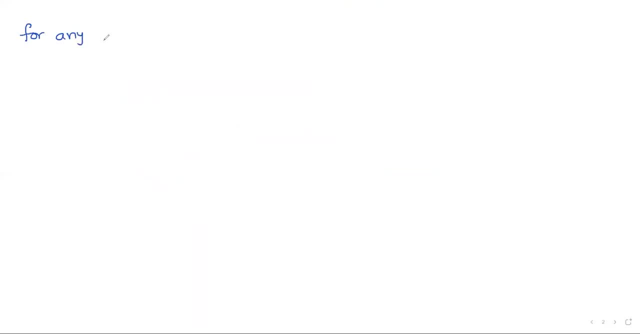 GCD of 0 comma 0 is equal to 0.. Now, finally, for any two integers, the Euclidean theorem is: for any two integers, a and b, GCD of a comma b is equal to GCD of b comma b mod a. 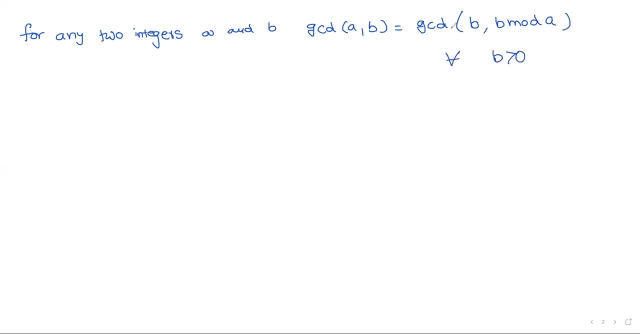 For all b greater than 0,. this is the Euclidean algorithm If you want to calculate GCD between a and b. finally, the answer is this: is This is repeated. Okay, Now, what is this? Apply the division algorithm. Apply the division algorithm for all a and b. Suppose. 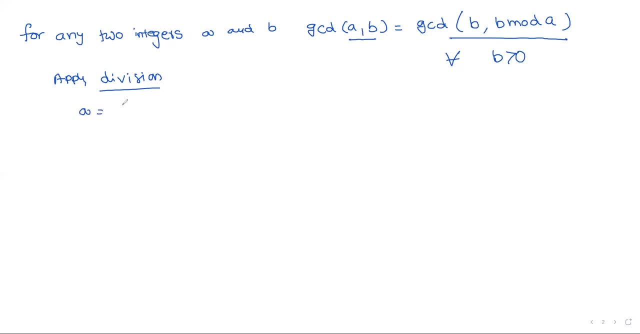 a is a number. It is represented in terms of: Q1 is the coefficient, B is the dividend. Sorry, B is the divisor, R1 is the reminder. Now, d is equal to what is the GCD? Simply GCD of b comma. 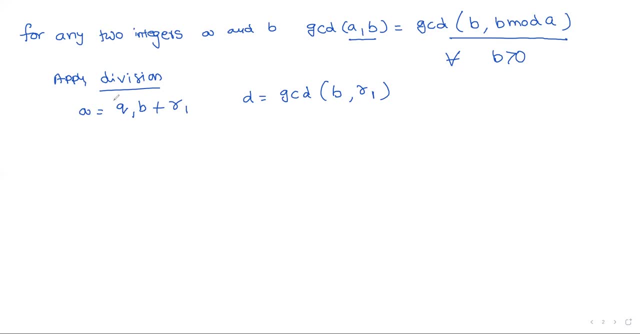 R1.. If you want to apply the same division algorithm multiple number of times In the next situation, apply for b comma R1. That means b is equal to. you can write like this: Q2 into R1 plus R2.. Now the GCD becomes GCD of next time. which value are considered? This is: 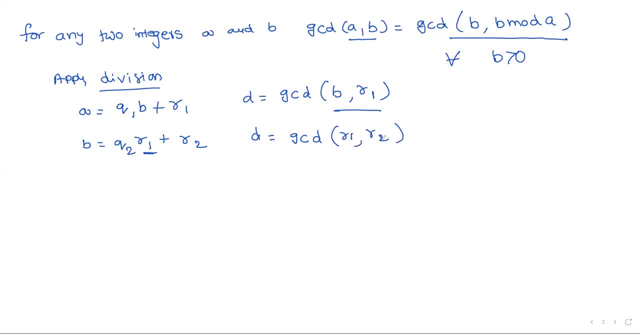 the divisor R1. and this is. You got it First time. A is the dividend, B is the divisor. In the next iteration, B becomes the dividend, The reminder- whatever the reminder we are getting- that acts as the divisor. The same operation, For example, if you require next: 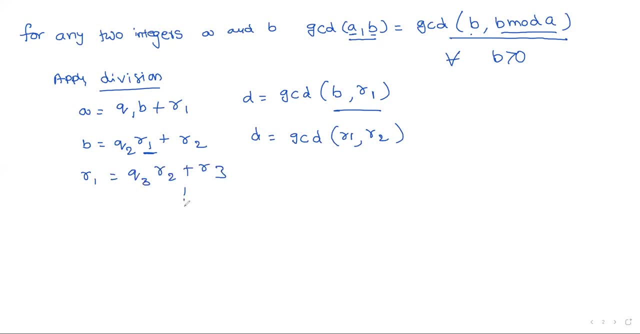 time Q3 into R2 plus R3 and so on. You can write any number of times. For example, Rn minus 1 is equal to Qn plus 1, Rn plus 0. At the final stage, the reminder is 0.. We are. 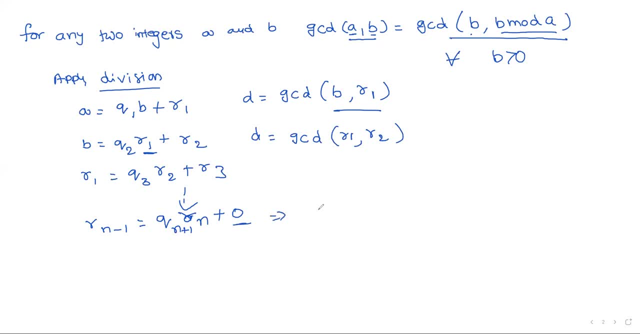 applying the process. So simply, for each and every iteration, D is equal to GCD of Ri comma Ri plus 1.. The operation is repeated until GCD of Rn comma 0.. The operation is repeated until the reminder is 0 and the final answer is Rn. Now, the same thing. what we discussed, the same thing. 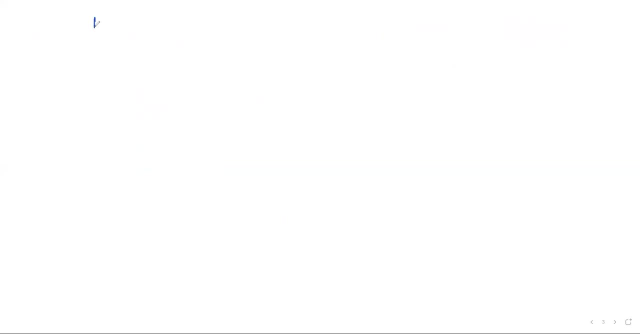 explained in algorithmic flow. First here, start the procedure. First check the two numbers, A greater than B or A less than B, For example. if A greater than B, what is happened? Simply, A is the largest value. Divide A by B And calculate the reminder. If you are dividing A by B, we are getting 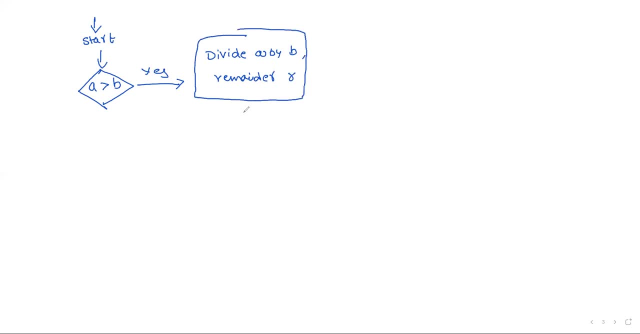 a reminder as R. This is the first step. Now, if the reminder R is greater than 0 or is not greater than 0, suppose if the reminder is greater than 0, assume If the reminder is greater than 0, in the sense the GCD is not at all. 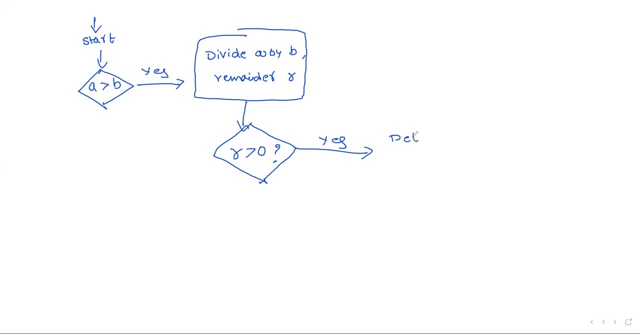 calculated. Simply replace A with B. That is, dividend is replaced with divisor. Now what do you have to think? Replace B with R. Whatever the reminder we are getting, replace B with R and apply the same process. This is the basic. For example, if A greater than B is false, then what we are doing Simply perform swap operations. Swap A- B. That means always we are dividing the largest number with the smallest number, and apply this procedure. 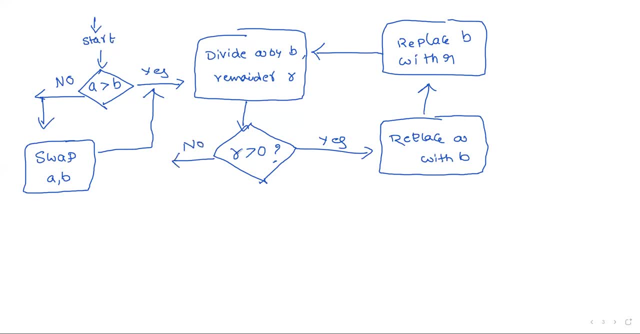 Suppose if no, no, in the sense reminder is equal to 0. And simply we give the result: gcd is the final value of b. The value of b is the gcd. end of the process. End of the process. This is the procedure to calculate the gcd. 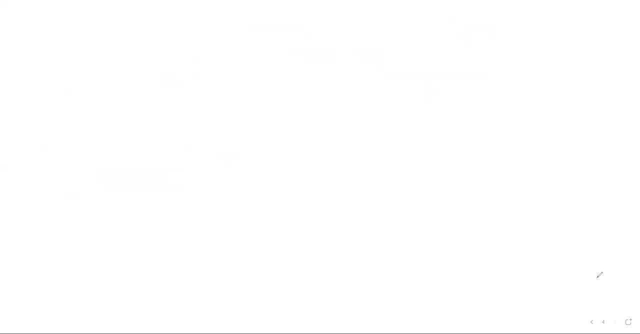 Now I will explain one blind procedure. How do you calculate the gcd of two numbers, For example 4 comma 3.. What is the procedure? This is the mathematical procedure. So 3, 4 jar 12.. The remainder is not equal to 0 again. 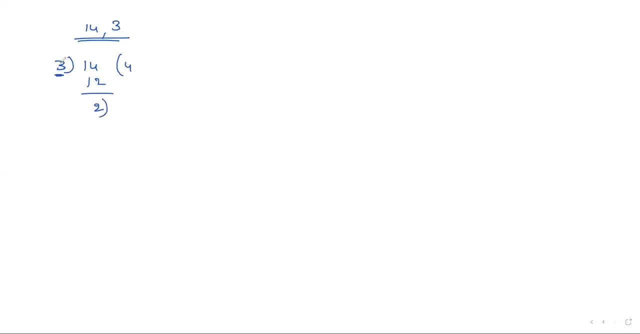 2 is the remainder. It becomes the divisor. Previous divisor becomes the dividend: 2, 1 jar 2, 1.. Again now the 2. 1, 2 jar 2.. The remainder is 0.. Whenever the remainder is 0, this 1 is the gcd of the two numbers. 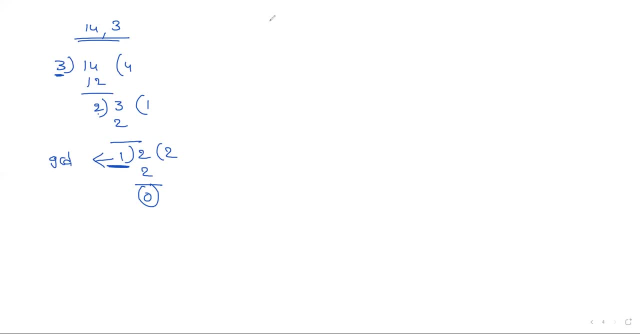 1 is the gcd of the two numbers. Now consider one more example. This is the gcd of 150 comma 35.. The same example. This is the example in terms of Euclidean algorithm. How do you represent? You have to represent: a is equal to q1 into b plus r1. 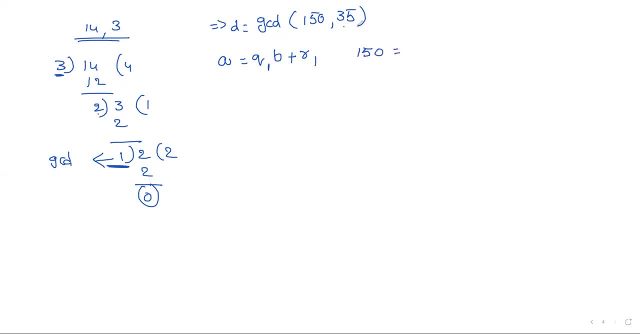 What is a? That is 150 is represented in terms of 35.. That is 4 into 35. Plus 10.. So here I will represent in this format also: That is 150t is divided with 35.. 35, 4 jar 140. 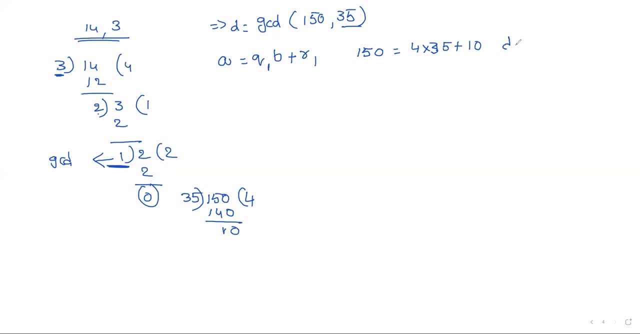 The remainder is 10.. This is the thing. Now repeat the process In the nested relation. 10 is the divisor, 35 is the dividend. That means 35 comma 10.. What is the Meaning of this one? Now b becomes q2.. 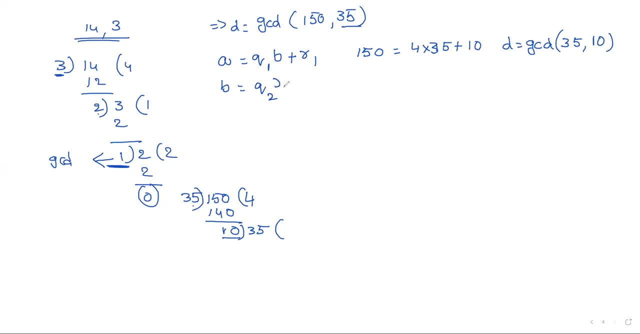 That is the coefficient. Whatever the coefficient, you are getting q2 into r1 plus r2.. That is, you have to convert this 35 in terms of 10.. So 35 is equal to 3 into 10 plus 5.. 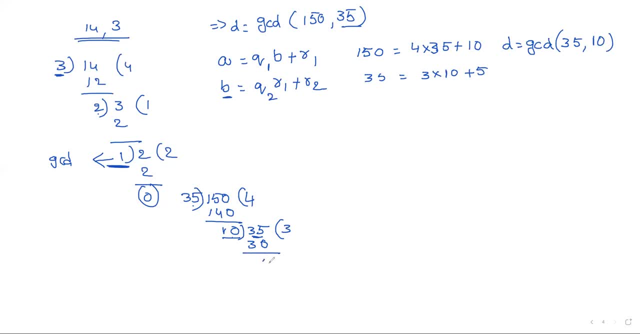 So this one 10 threes are 30. The remainder is 5.. In the nested relation, d is equal to gcd half. What is the coefficient? we are getting 10.. So 10 becomes the dividend. And what is the remainder?